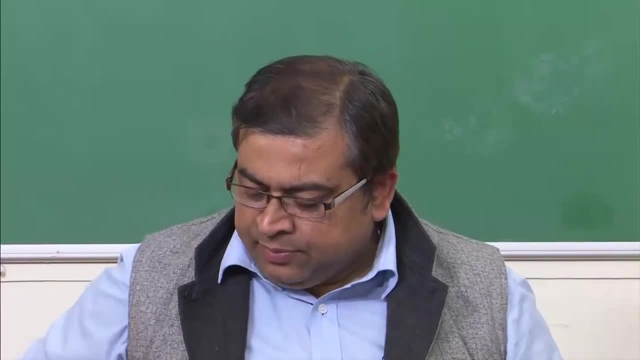 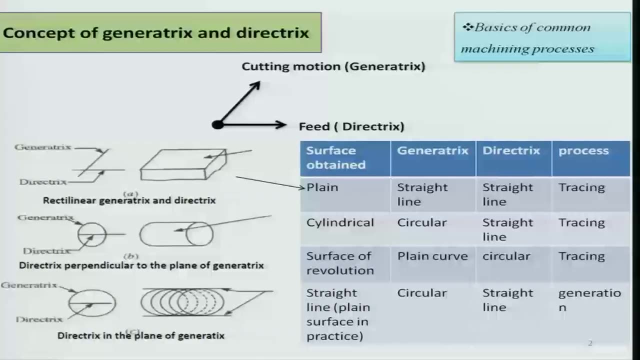 the tool moves with respect to the workpiece, And this slide right here shows the concept of two important motions associated with the motion of the tool with respect to one workpiece. One is the feed motion, which is actually also known by the term directrix, and the cutting 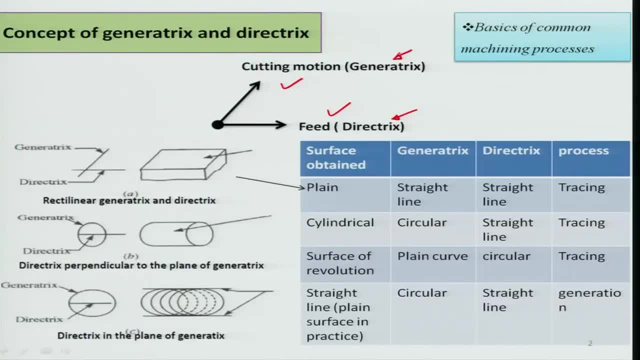 motion, which is basically the generatrix. So, as the name indicates, the different geometries that are expected out of machining processes are formulated by a manipulation of the generatrix and the directrix. For example, let us say, in case of a shaper machine or a plane machine, there is a movement of the tool. with respect, 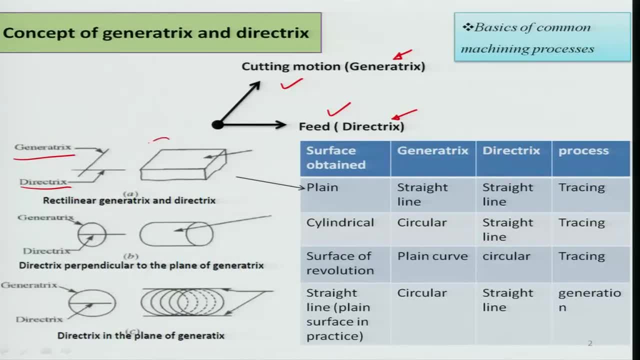 to the workpiece, which is mostly on an x- y plane. So this slide here shows the reclinear motion of the feed direction and the cutting motion, and they are perpendicular to each other, making you know a 90 degree angle. And so, therefore, 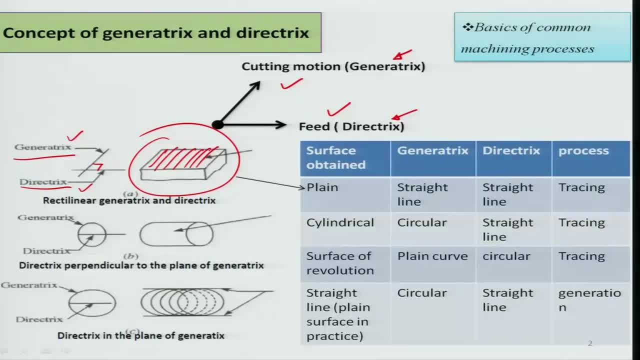 you can have a x- y plane generated because of such directrix and generatrix, both straight lines perpendicular to each other. So we can obtain a plane surface out of a straight-line directrix and a straight line directrix, and the process can also be known as tracing. 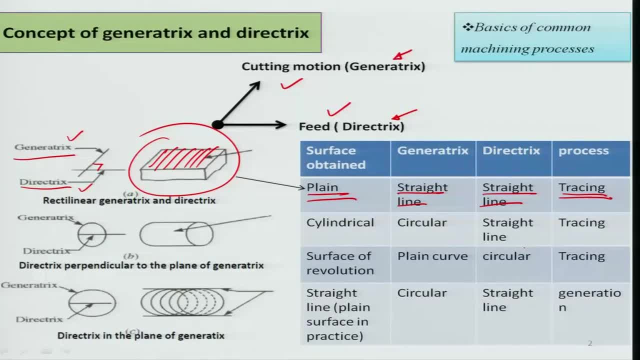 Similarly, in the case of a turning center, you have normally the motion of work piece in a circular manner and we can say that the generatrix direction of the cutting motion that happens is in a circular manner and the relative feed direction of the tool with respect. 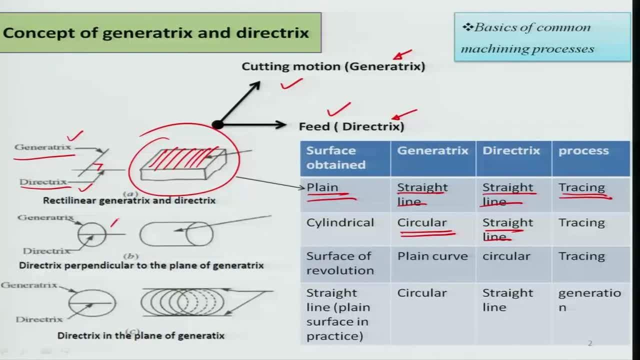 to the work piece is again straight line. So a straight line in a circle in generally will yield or which make an array which is like cylindrical in shape. So of course the straight line is in a direction perpendicular to the direction of the cutting velocity. 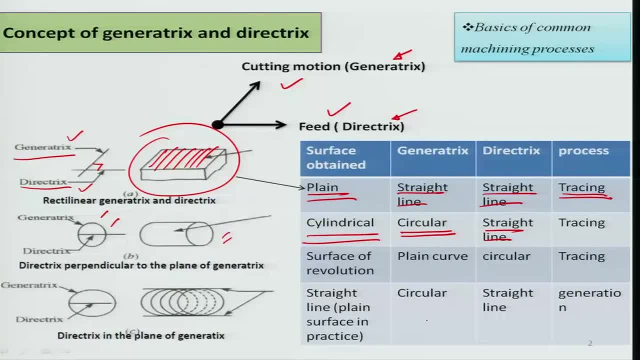 So that is very important, particularly here or in case there is a motion which is related to circular motion. So the circular motion of the tool and the motion feed, motion of the tool in the direction almost in the same plane as the cutting velocity or towards the direction of the cutting velocity. 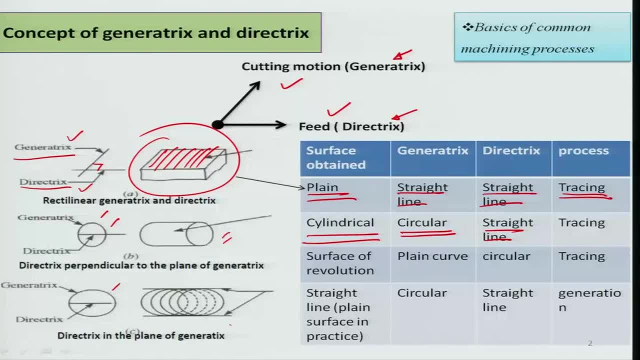 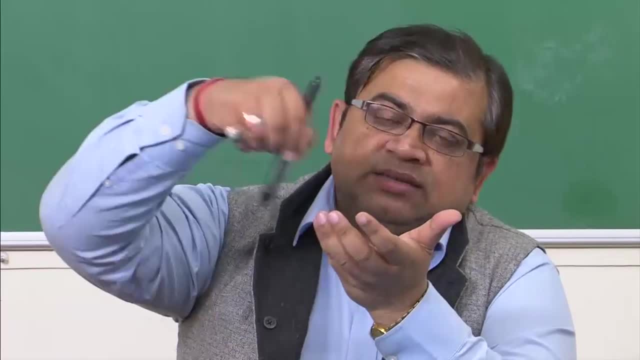 in that case also, you can generate a plane surface. The example of that is milling. So in a milling system you have, let us say, a circular motion and the cutting motion is really along a circle, and the cutting velocity and the way that the chips get formulated. 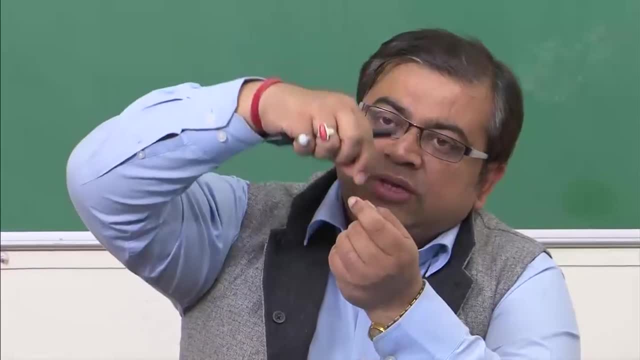 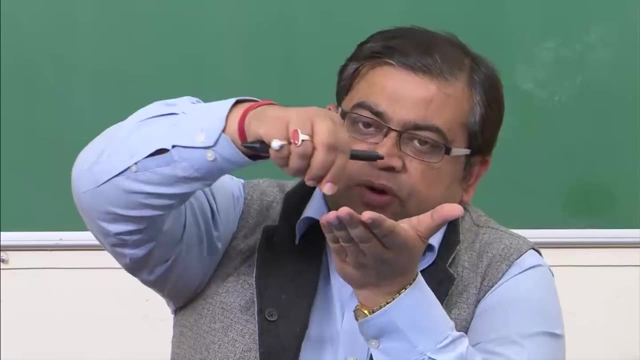 is So the question which can be asked is that, particularly in a face milling operation, is how the tool engages in a circular manner at different points. It is a multiple cutting tool, point cutting tool, So that you can have chip formations along that circle, and 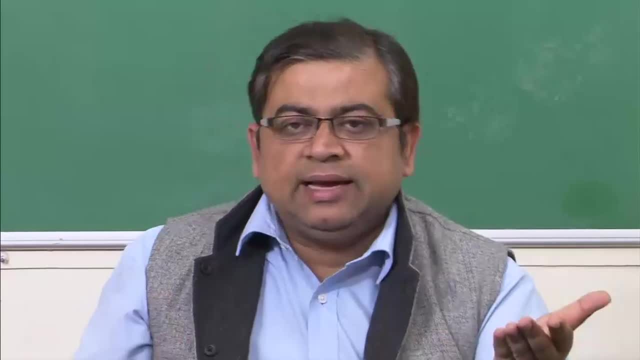 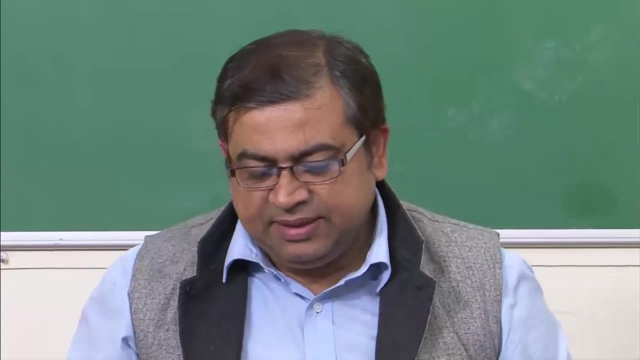 then you basically moving it in a direction, either perpendicular to the of the direction of the cutting velocity, And so you get a plane surface based on these two motions. So various complex geometries with different symmetries can be obtained with trying to. 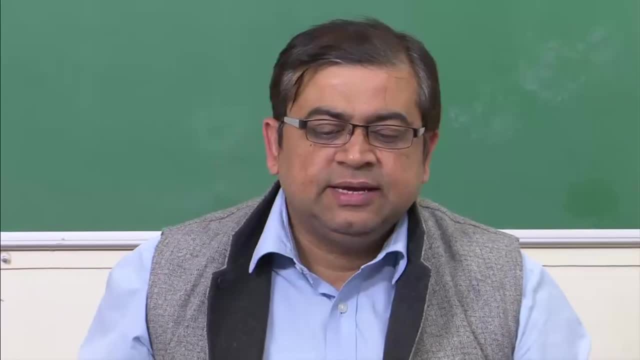 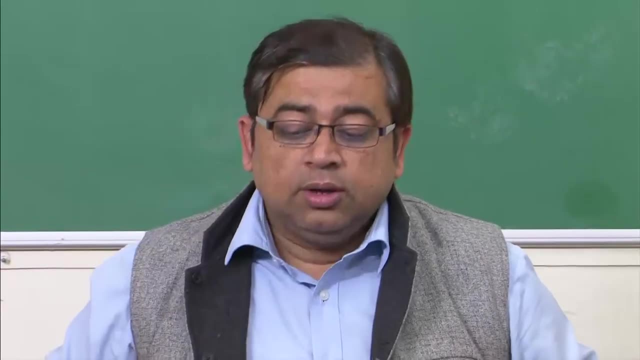 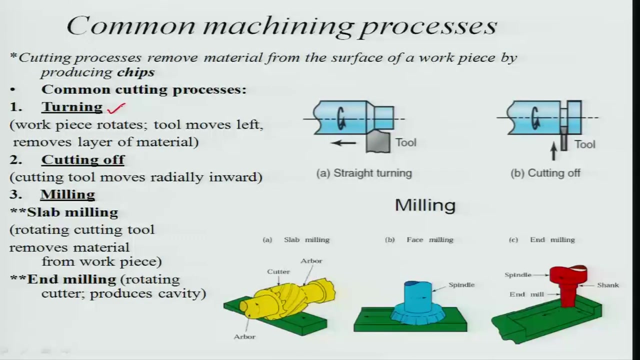 with different cutting motion directions and feed directions, and that is how you understand the basic engagement of the tool process with respect to the work piece. So let us talk about now some of the processes. So we have the example of turning where the work piece rotates and the tool moves to the left direction. you can see here that the tool 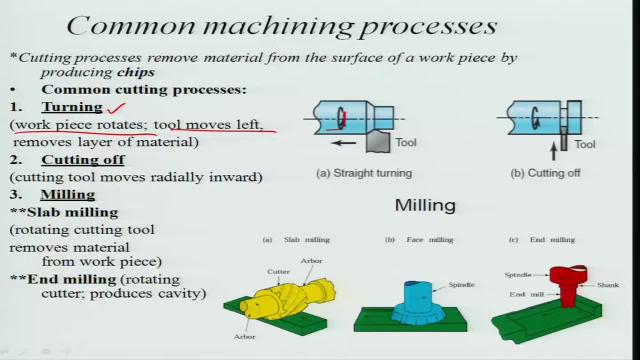 is moving in that perpendicular to the direction of the cutting velocity, which is actually tangential to the circular motion here, and this generates cylindrical surface, as we had earlier illustrated. So this is the case of straight turning. there is a cutting off. So basically, this portion is now being shaved off using a cutting, a parting tool, So the 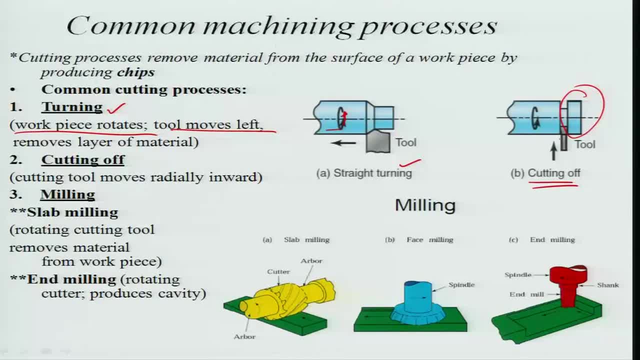 surface is completely eliminated from the cylindrical surface, So cutting tool moves radially inwards. You have a Again milling, which is another form of cutting in slab milling operations. you have a rotating cutting tool and it removes the material from the work piece as shown here. The milling 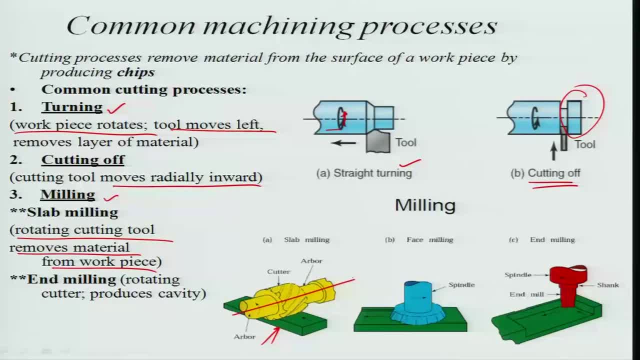 tool is typically mounted on to an arbor, which is a axis which provides rotation to the cutter and the work piece is moved. actually, perpendicular to the work piece is moved in both x and y direction with respect to this particular cutting motion. So this is the case of the 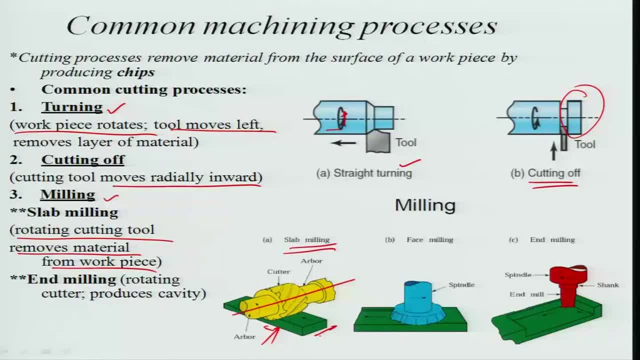 milling function, and such examples are known as slab milling. You can also have different other forms of milling, like the face milling example that I was providing, where the cutting motion is also along a circular plane, which is probably in the similar direction. So the cutting velocity, for example, in this particular direction is similar to that of 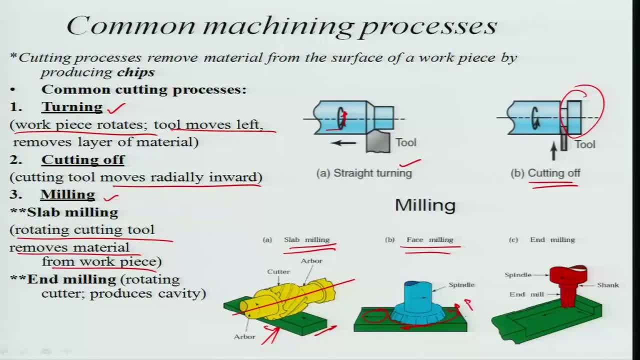 the feed motion or is similar again to the direction of the feed motion of the tool in the y direction. So in these particular examples you can have a planar surface. Then you have have end milling operations where you can actually have a rotating cutter and it produces. 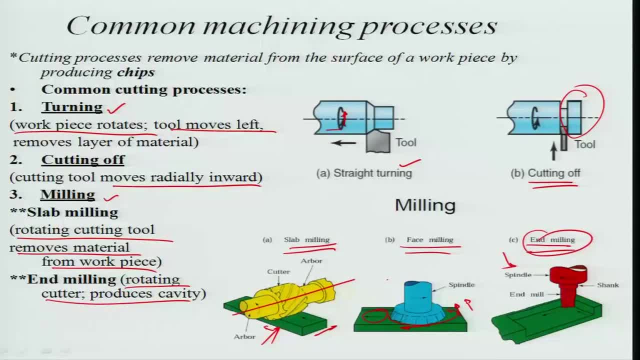 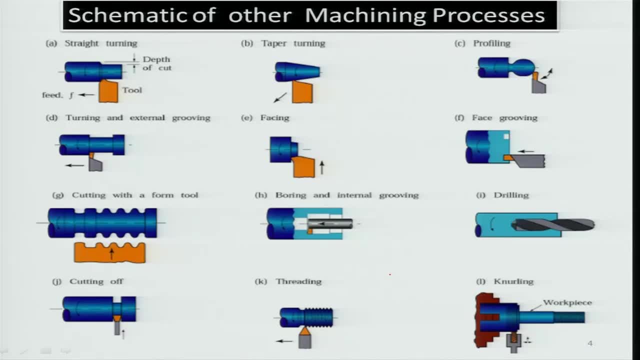 a cavity, as you can see here right about here. So these are different variants of milling process, some other common machining processes, particularly for turning. you can have a lot of different operations for straight turning shown here. there is a taper turning where the tool goes from in a tapered manner with respect to the rotating axis of the work piece. 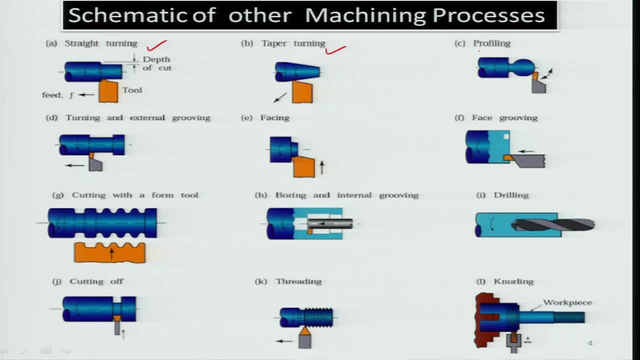 and it generates a profile. identical to it is motion. you have profiling, where you have a certain shape- x, y, shape- which is typically the curve of or the path that the tool follows with respect to a turning work piece, So that you can have a complex shape profiled. 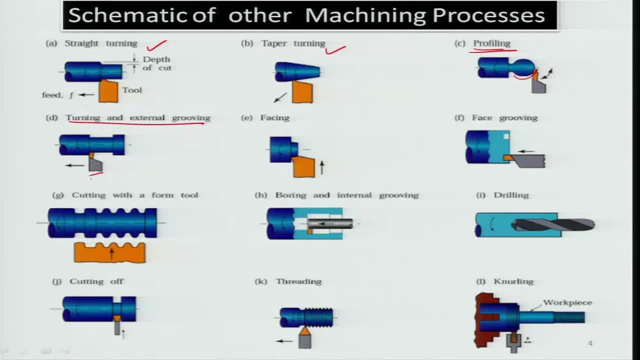 on to the work piece. you have turning and external grooving. as can be indicated in the highlighted here, you facing operation where one portion of the- you know circular work piece is completely removed or shaved off. You have a phase grooving operation where, by a different orientation of the tool, with tool moving in a direction perpendicular to 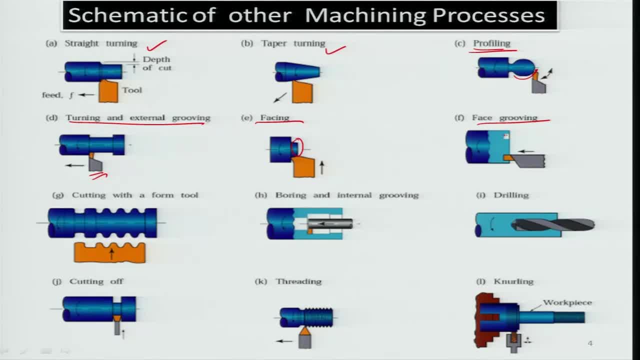 the circle of motion, you can actually have a small groove, as you can see in this particular example. this shows that of a cutting with the form tool. So you have exactly Something imprinted- the negative of something imprinted, of which the tool is shaped up to. 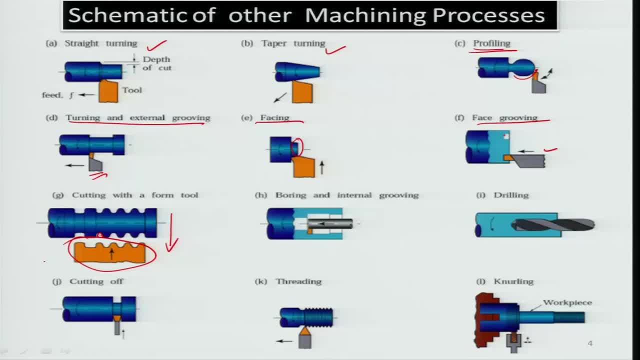 and so you can actually have a shape imprinted directly by cutting it with the form tool. You have boring and internal grooving, as illustrated here, which is typically done by a boring tool mounted on one of the spindle axis of the, which is sort of coaxial to the. 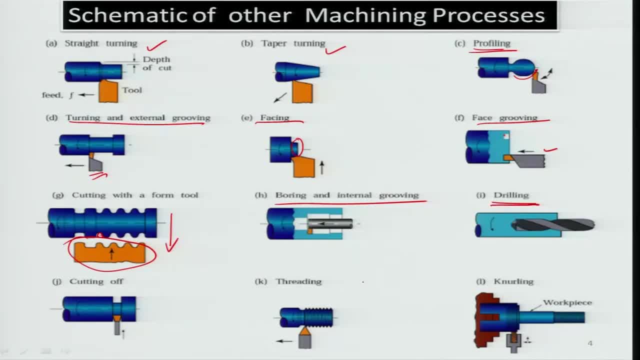 work piece direction. you can do in a similar manner by using a drilling tool. you know to drill on side of the cylindrical work piece. you can do cutting off by having a tool which would be enabled to go in a direction perpendicular to the radial direction with respect to the 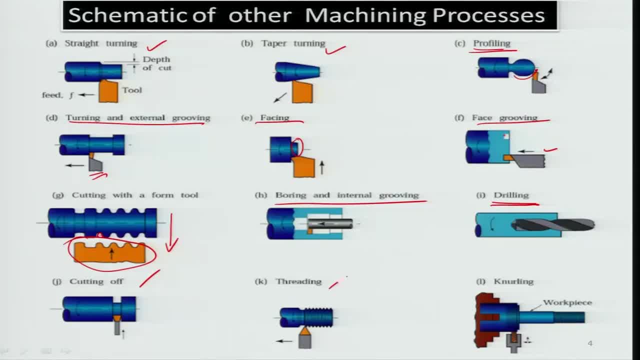 work piece and produce a deep cut. You have threading tool where the thread moves. the threading tool moves at a certain feed and it generates Threads, Threads of a defined pitch because of the motion of the tool in a direction parallel to the axis over which the work piece is rotating. 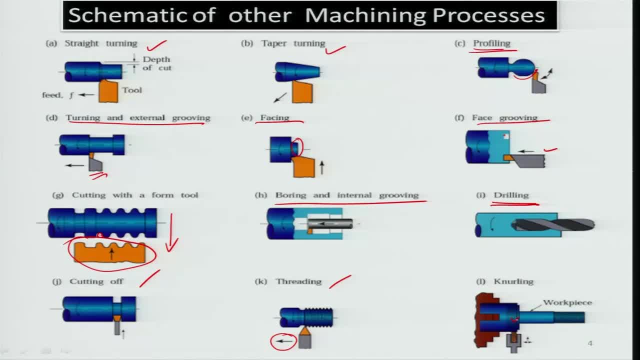 You have a knurling tool where you have a pattern impregnated on to the surface which is exactly the negative of the pattern that the tool contains. So these are different operations that you can actually use the turning system or lathe to obtain. 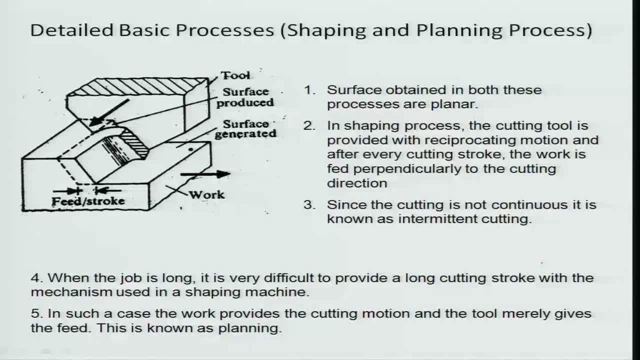 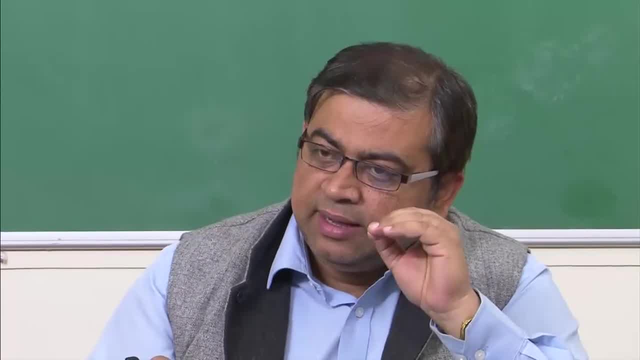 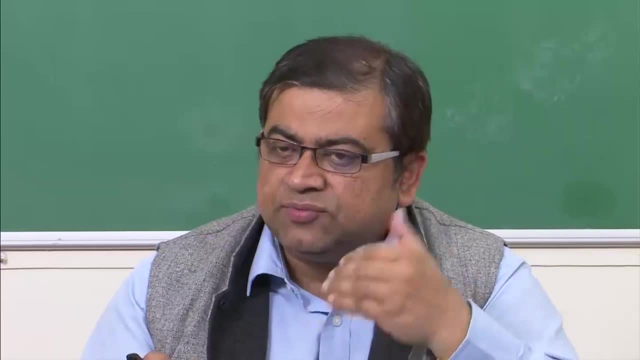 So if we talk about the basic processes of machining, It is really about peeling off of the material. So, as I told you earlier that there is a metal tip which would be engaged with another metal which is the work piece In our case, the metal tip is harder in comparison to the work piece and it actually plows into 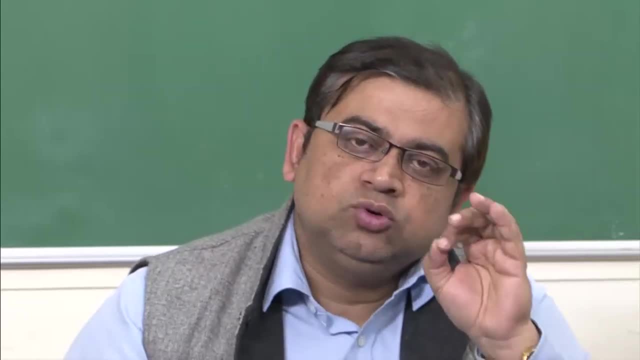 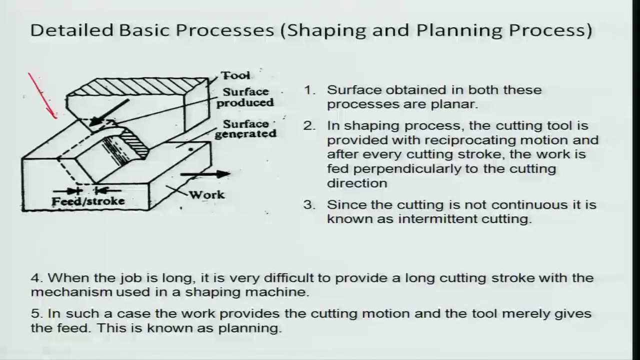 the metal and starts to peel off the metal. That is how you do conventional machining, or that is how the chip formation takes place within the system. So if I look at this figure right here, it talks about a basic shape Shaping or a planing process where the surface obtained in both these processes are planer. 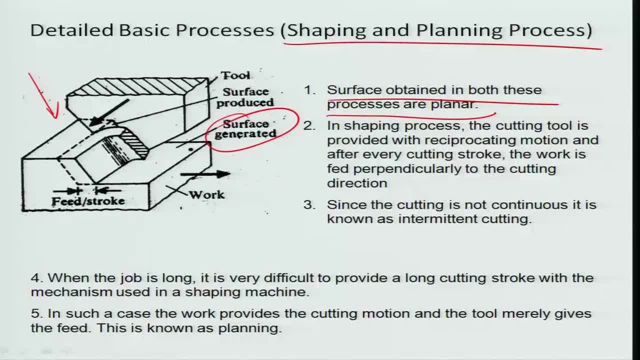 in nature. This is the cut surface, the surface generated. you can see here in this portion of the figure, and you can see how the peeling of action is happening at the point of engagement, of the cutting edge of the tool, which is actually this edge right here with respect to the work. 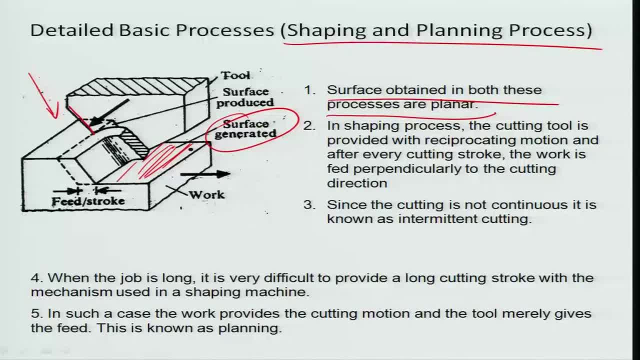 piece. So you are having a portion of the work piece which was otherwise making this particular substrate or surface Or constituting this particular surface, cut off so that you have a similar surface produced at the bottom here and there is a certain feed at which you can move this tool inside. 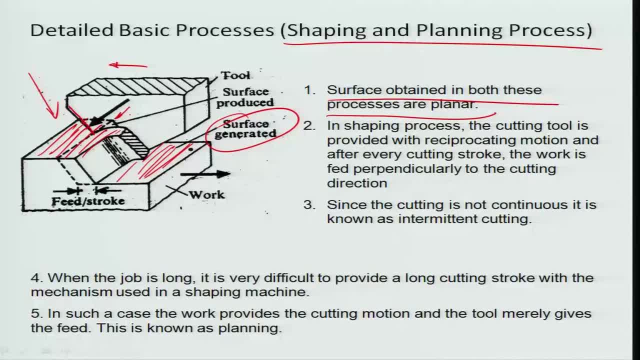 whereas moving it at a certain feed velocity, perpendicular, and so that is how you generate a x? y surface of the work, you know, corresponding to the different feed and stroke. So you have a tool and you have a surface which is produced. So, in shaping process, the cutting tool is provided with reciprocating motion and every 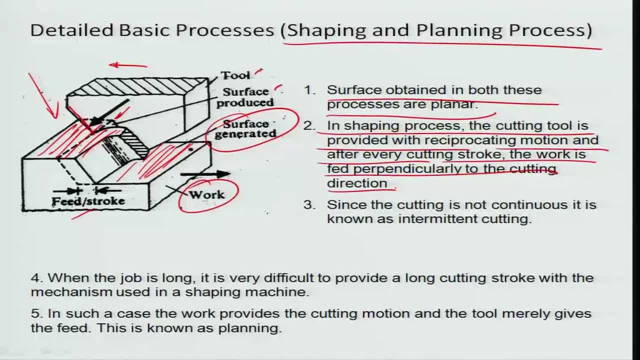 cutting stroke, the work is fed perpendicularly to the cutting direction. Since the cutting is not continuous, it is known as an intermittent cutting process. it is not similar to that in the lathe machine, where you have a continuous flow of chips coming out When the job is long, and it is very difficult to provide a long cutting stroke with mechanisms. 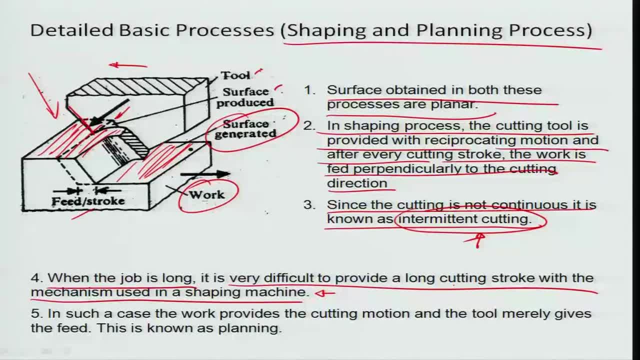 used in a shaping machine. generally, in that kind of a case, instead of moving the tool all over to the whole span- Similar to the whole span of the job- you basically move the work piece. So the work piece provides the cutting motion and the tool merely gives the feed, and that. 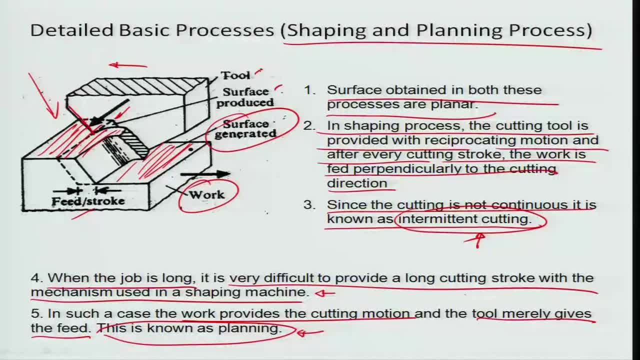 operation then would be known as planing operation. So only difference is in terms of the work piece size and what moves. So the primary cutting motion would be generated by the cutting stroke of the tool if it is a smaller component and the operation then there in would be known as shaping. 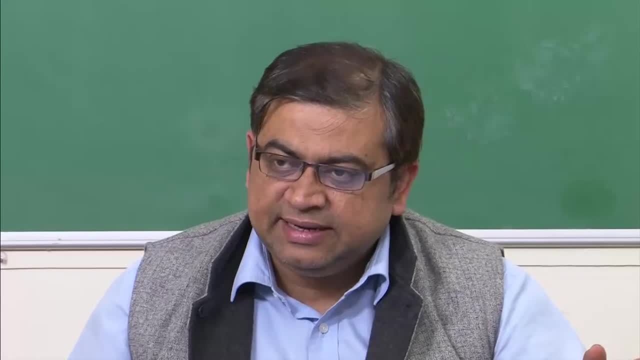 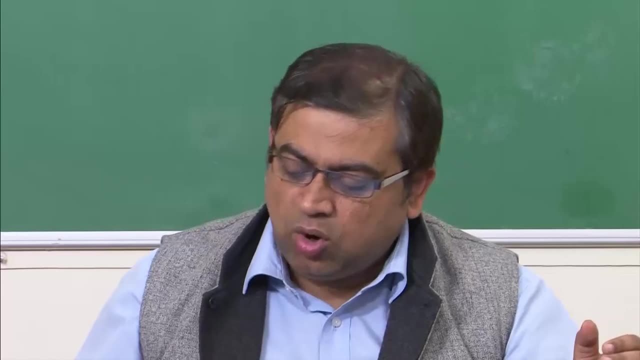 And vice versa. if the work piece is the one which is generating the cutting motion, whereas the tool is only giving the feed and it is a, let us say, a long longer or a larger component, then that kind of a motion is now known as a planing motion. 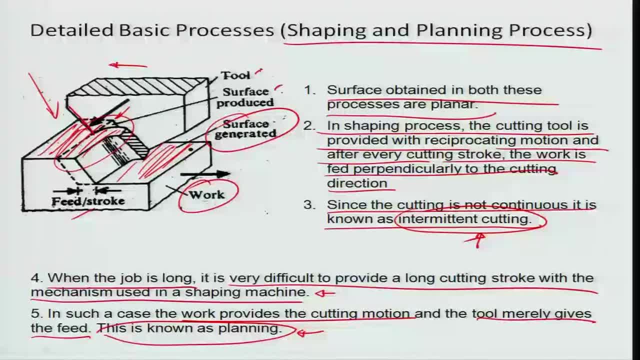 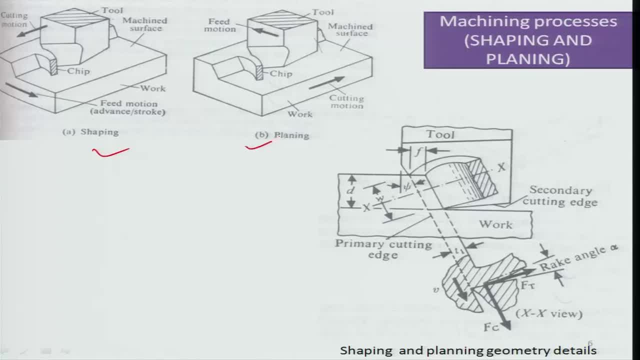 So, but effectively what you can see is the peeling process which is going on. here You have similar examples where the same- this is shaping and planing- happening. in both the cases you have peeling off of the work piece which is happening And you can actually do a mechanistic diagram here which I am going to illustrate later. 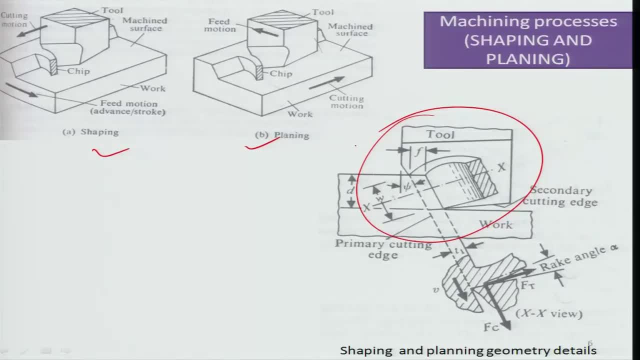 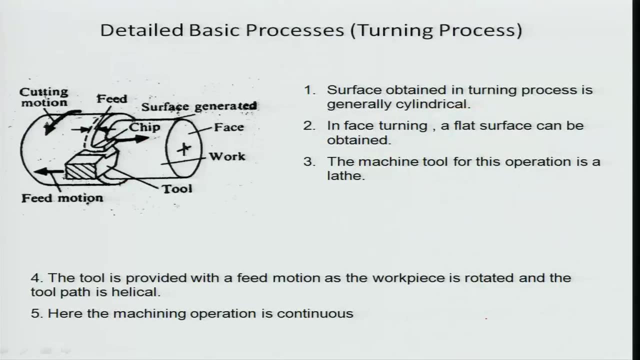 where we can see how the chip etcetera is generated, you know where the function of the rake angle or different other forces, like the cutting force or the friction force which comes in there. So similar kind of a process of peeling can be illustrated, even for the turning operations. 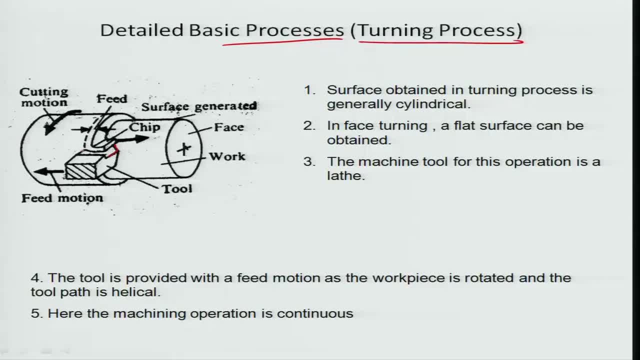 So here also you can see a tool and you can see the level of engagement of this tool with respect to this tools work piece. So this is a tool surface or tool edge which then peels off the material, the surface material, and it basically tries to again remove the material by peeling action. it is a continuous 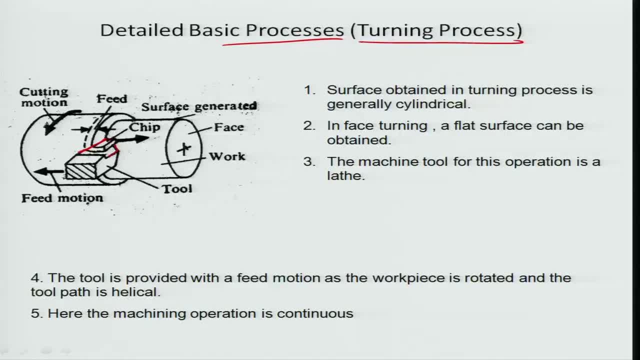 process again, because when the surface is rotating with respect to this edge, there is a continuous removal of the chip material from the work piece surface. So the substance surface obtained in turning process is generally cylindrical in phase turning. So this can be obtained. the machine tool for this operation is a lathe and the tool 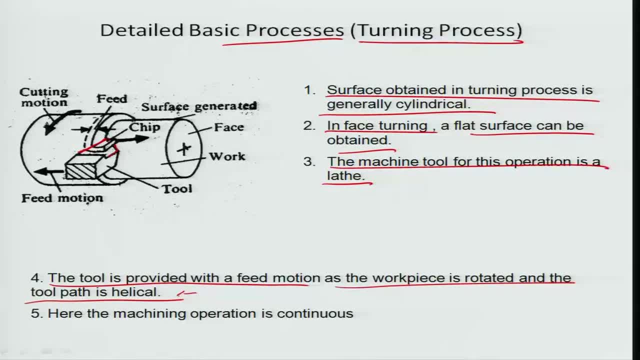 is provided with the feed motion as the work piece is rotated and the tool path is a sort of helical path that it follows for removing of this material. here you can see this is the surface which is generated because of the cutting motion and this was the surface. 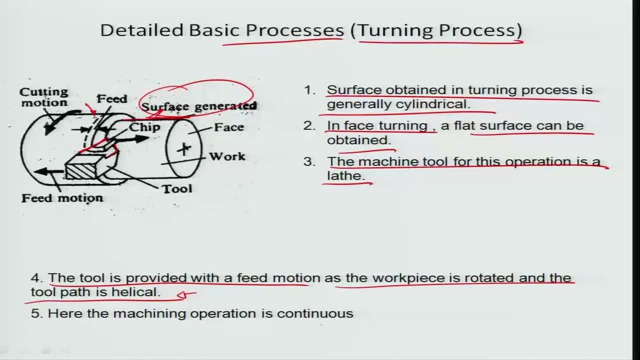 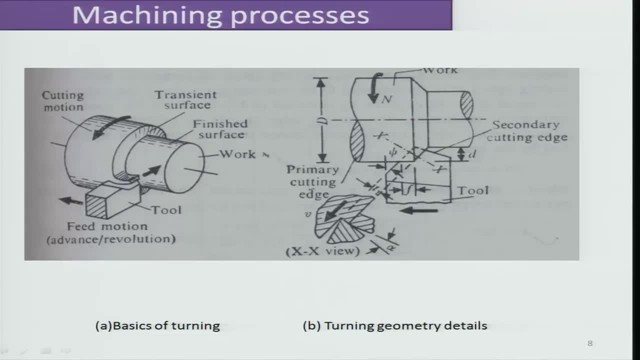 which was before, which is being cut to generate this surface, this new surface. So here the machining operation is a continuous machining operation. you can see how, again, the chipping action happens here, as a function of the different forces and the angles, And we are going to do all the analysis of how this chipping action happens in a later 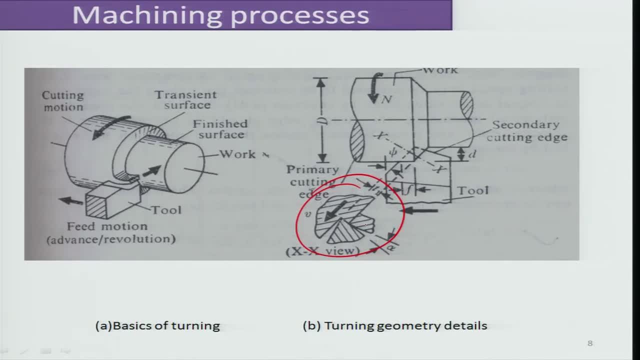 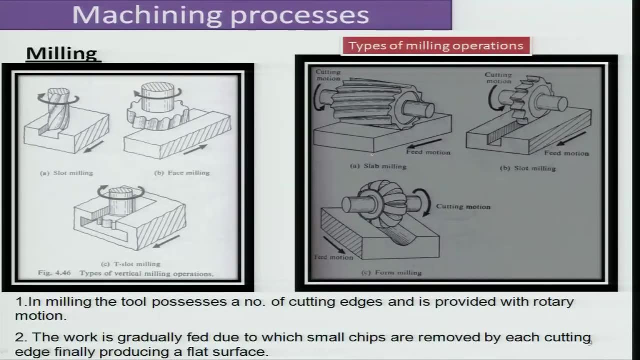 on stage, but that is how the basic of turning process happens. You have a similar kind of a strategy for milling processes. here, for example, you are seeing three different kind of millings. one is a slot milling, another is a face milling, another is a T slot milling, and I can see here that the there are different other kind. 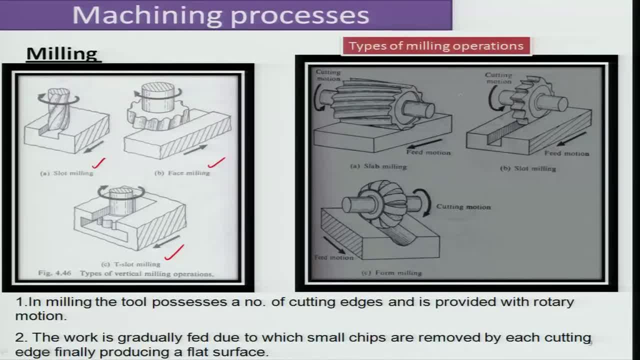 of millings. for example, in slab milling case, you can see that the milling tool is mounted on an arbor and there is a feed motion of the work piece. Similarly, there is a again another kind of a slot milling case, here with the similar. 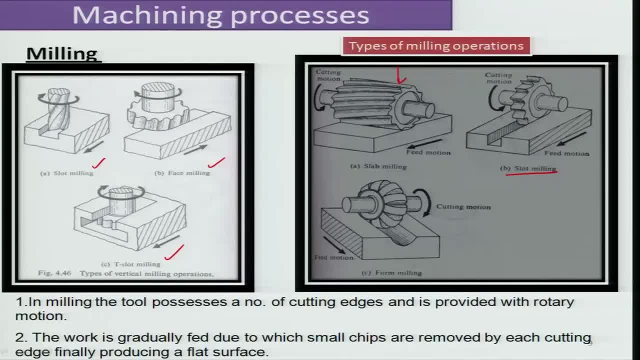 kind of a vertical, you know, mounting of the milling cutter or a form milling where a certain form, So a shape, is impregnated on to the surface because of the form of the tool which is there. So the same operation of a rotating tool, you know, which is a multipoint cutter, is being 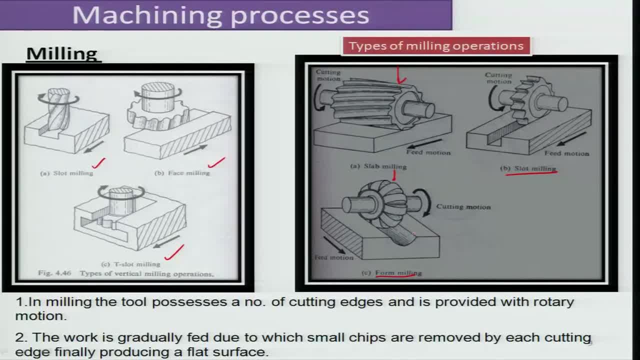 utilized in various forms to obtain different kind of peeling operations, as the milling system. So in milling the tool poses a number of cutting edges. it is provided with a rotary motion. the work is gradually fed, due to which small chips are removed by each milling tool. 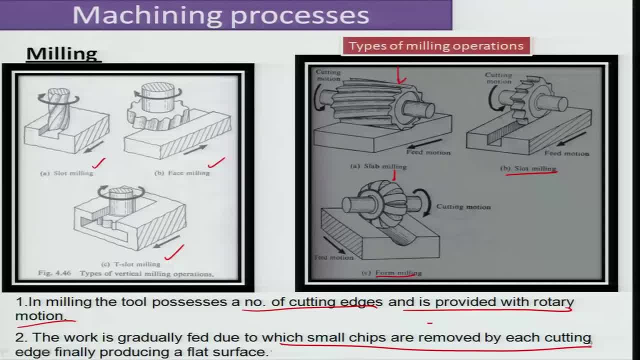 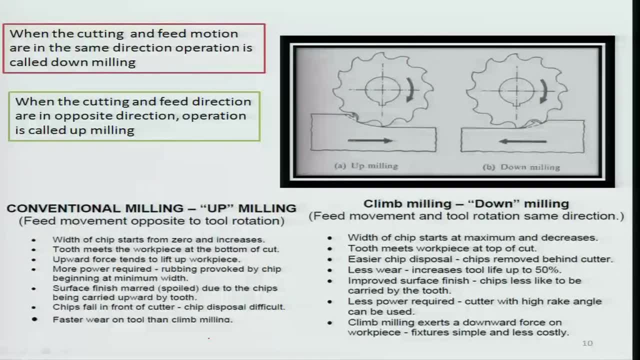 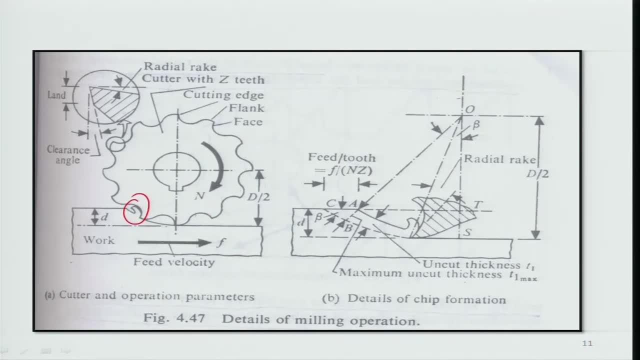 And finally it produces a flat surface. So but then again, if I look at the way that this milling operation is performed, it is really about the way of that peeling process again which is happening somewhere here. So if the engagement of the cutter happens at a portion somewhere, here there is a original. 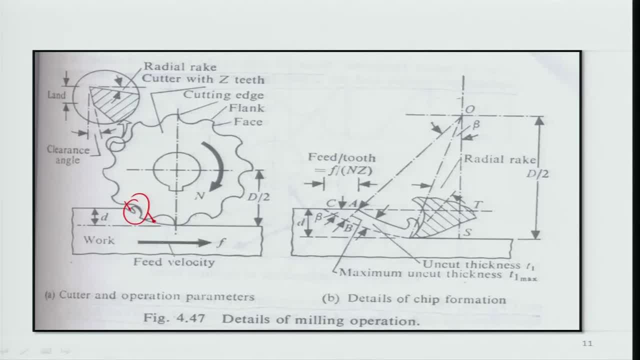 surface which was actually this surface, which is been cut of now into this new secondary surface and there is a milling cut, the chip which is coming out because of the engagement with the cutter So effectively. again it is the same peeling.